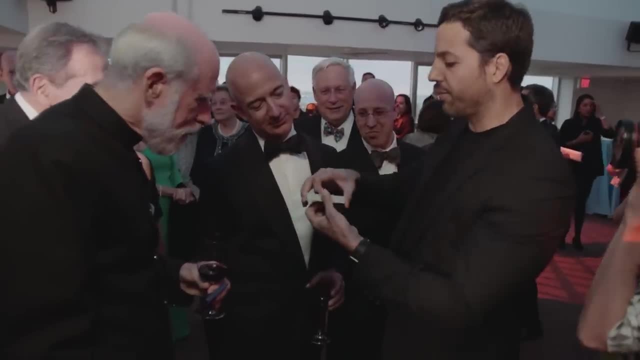 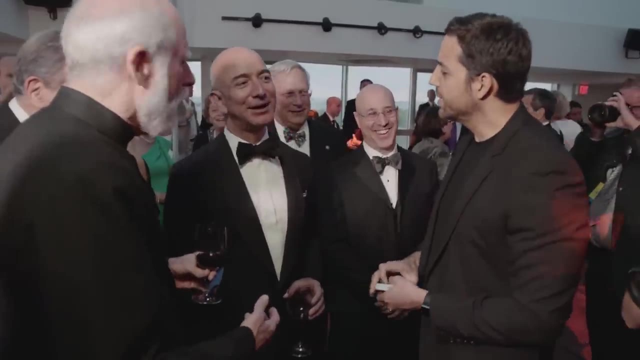 See that obvious bend in the card. Yes, there it is. These go above. if I just hit, See how it pops up and through the deck. But, Jeff, let me see. We need a high-speed camera. But, Jeff, you can do it. 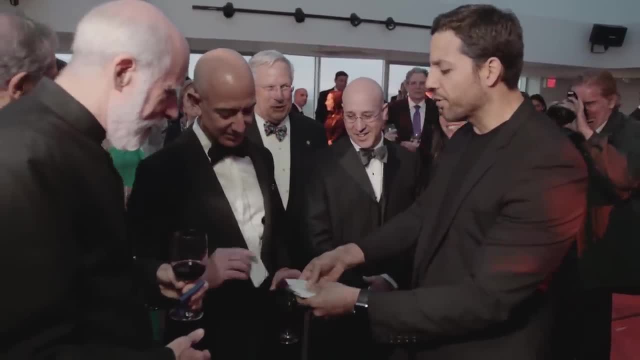 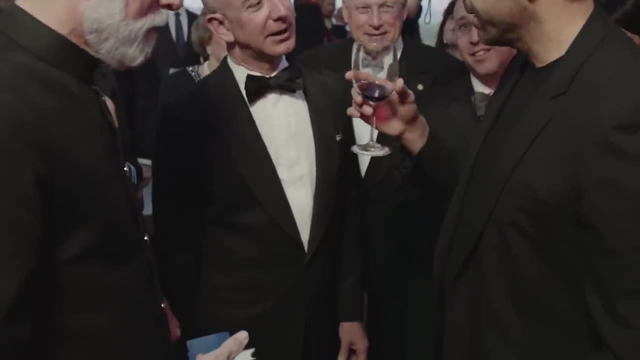 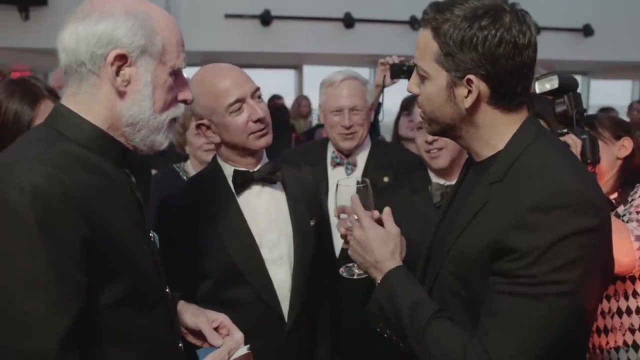 Take one out, Whatever you want Of all the cards you're going to have. which one is it? Do you mind? Sure, Is that? okay? Yeah, yeah, This is your glass. Yeah, this is your glass. Jesus, what are you doing? 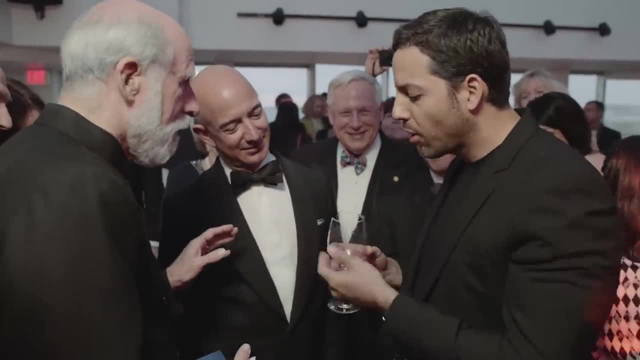 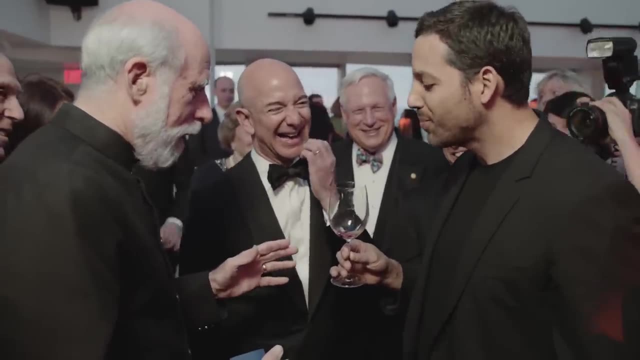 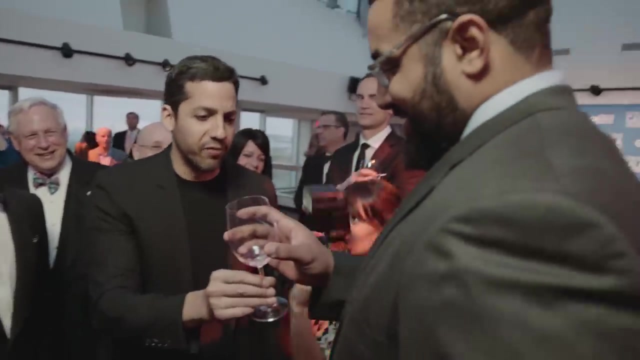 I'm going to get some safety goggles next time. How is it You make sure that's actually real glass And be careful Don't hurt your hands. Just cut your hand there, That'll be fine. That's real glass. Oh, back to what we were doing, though. 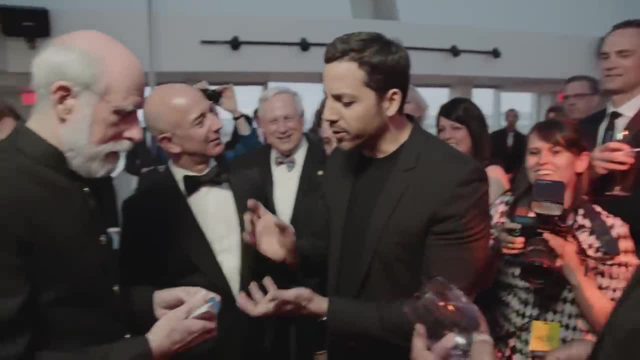 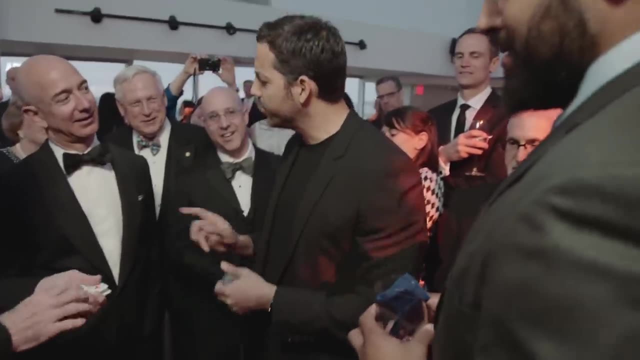 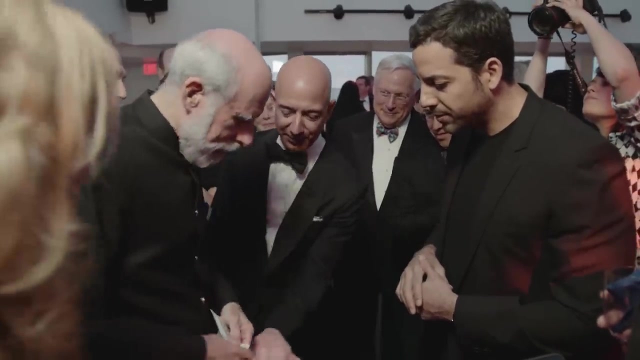 Could you shuffle? I'll take the napkin so you have a free hand. If you can mix, And who has an eye? I do. I have an iPhone. Do you have an iPhone? Perfect, let's use his. It's very difficult. 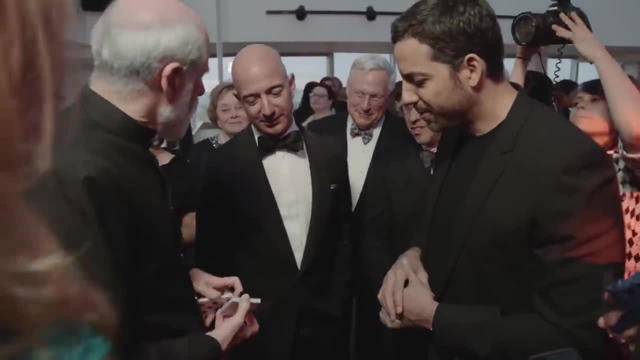 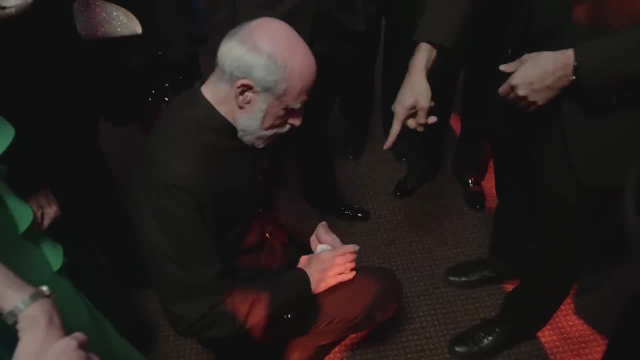 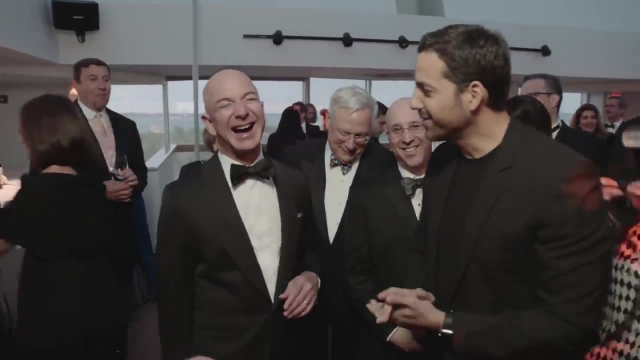 You need a table. Laura can do it, Like Vanna. That's a good shuffle. Maybe do another one, though. Oh, you know what If we could eliminate that? I don't want anybody to get hurt. Okay, That looks good. 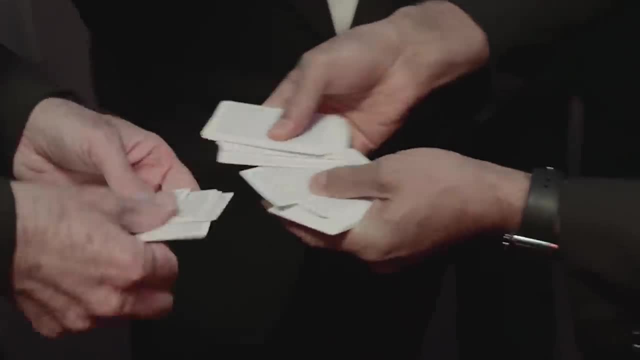 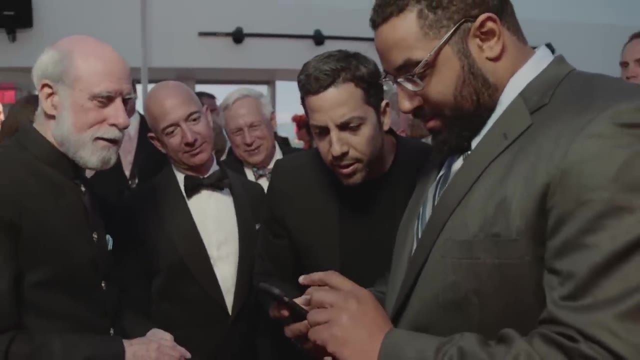 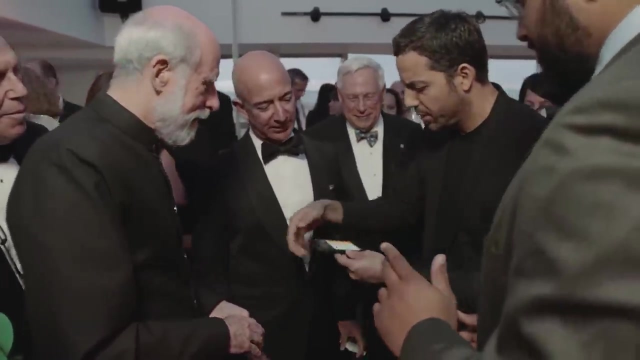 So take a poker hand from the deck. Okay, perfect, Can I do this? Can you open up the calculator app on your phone? Yes, it is. Oh yeah, perfect, Great, perfect, Good, good, good. Can you take this first? 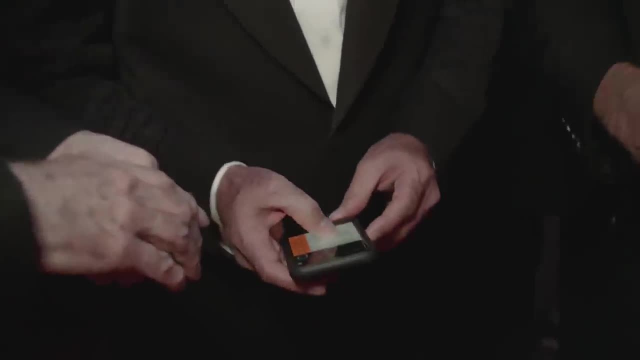 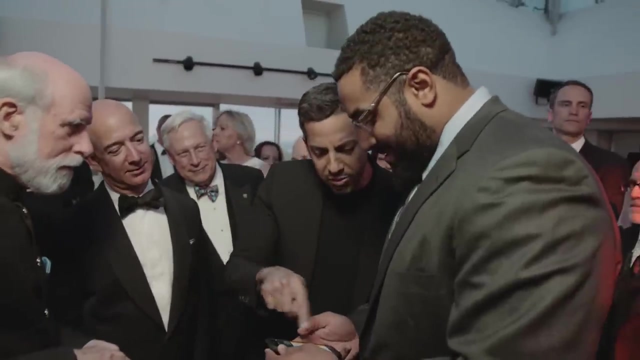 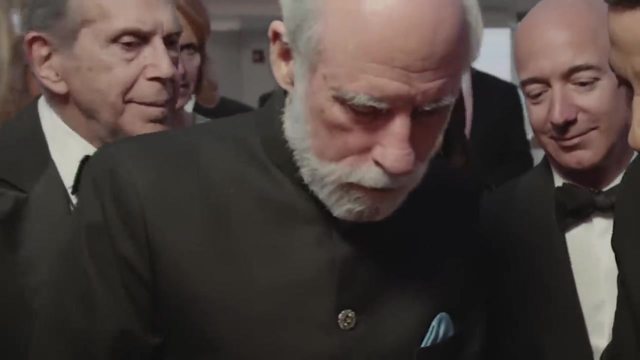 Can you type a three-digit number for me? Any three-digit number, Do times. Can you take it, And I know you're a mathematician, so do like a three-digit number. Two plus. Can you do this? Do a number.